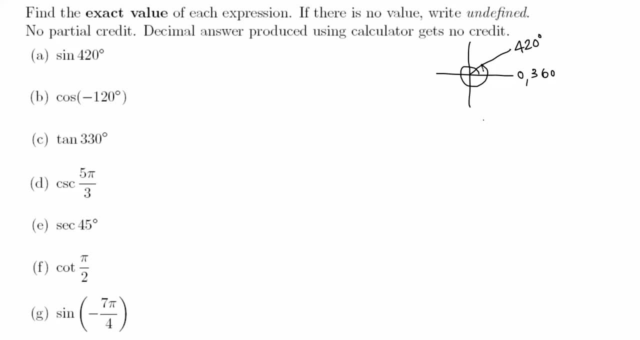 that's in the first quadrant. Okay, so in first quadrant all trig functions have positive values, so we get positive of sine. the reference angle here is 360 plus 60, 420, so that's sine 60. And sine 60 is root 3 over 2.. Next cosine of negative 120 degrees And we: 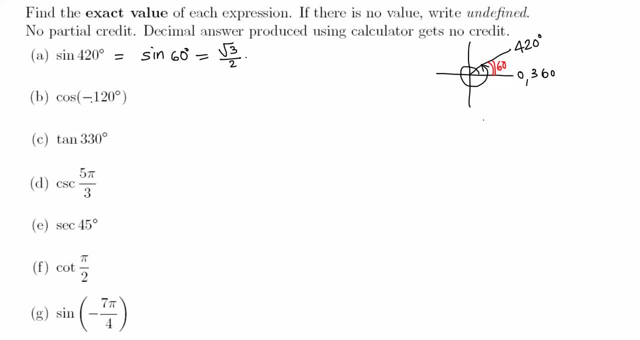 know that cosine is an even function. So cosine of negative angle is same as positive. cosine of that angle 120.. Now 120. That's 180, 90.. so 120 degrees is obviously in second quadrant somewhere. okay, 120, let's find. 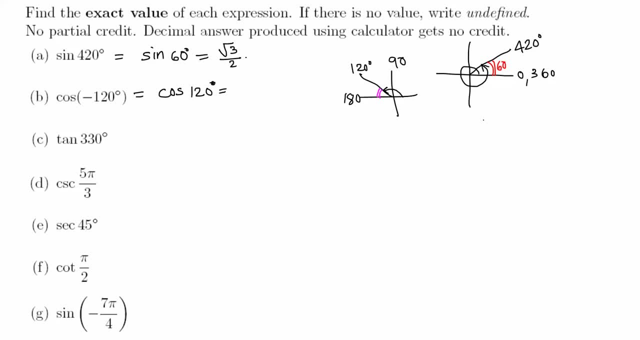 the reference angle. so 120, 180. so this will be 60. so in the second quadrant from the quadrant rule all students take calculus. only sine and its reciprocal have positive values. so cosine has negative value, cosine of reference angle that's 60. negative cosine 60 is 1 half. the value of cosine 60 is 1 half. okay, 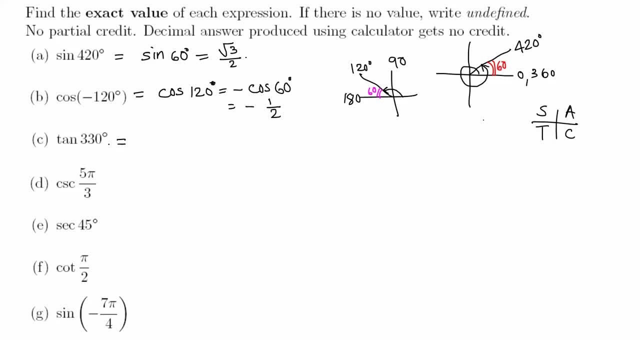 Part C, Tangent 330, now 330 is in, so this is 0, or 360 270, so 330panels is half. We havegamov Workbook. Sam made moreôn zero or three, and so Breakdowns: 토 Nove Oteroो, imperial Standard English. 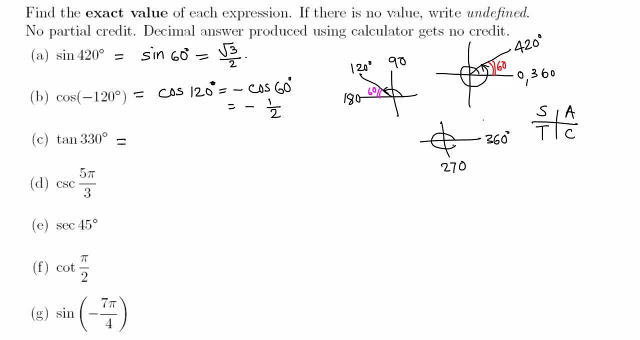 降 in the following words: infant stress test. stainless steel, porcelain, and is in fourth quadrant somewhere here. that's 330. so this remaining 360 minus 330 is the reference angle, that's 30. okay, so that's tangent in the fourth quadrant. fourth quadrant, only cosine and secant have positive values, so tangent. 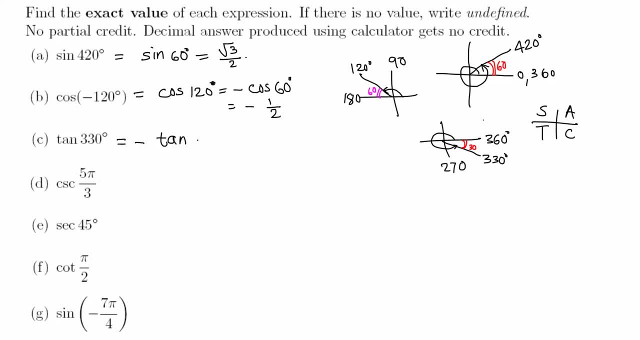 has negative value of tangent reference angle 30 minus, and the value of tangent 30 is 1 over root 3. okay, or you can rationalize this and get: multiply top and bottom by root 3. you get root 3 over 3. but this is good enough, okay, cosecant. 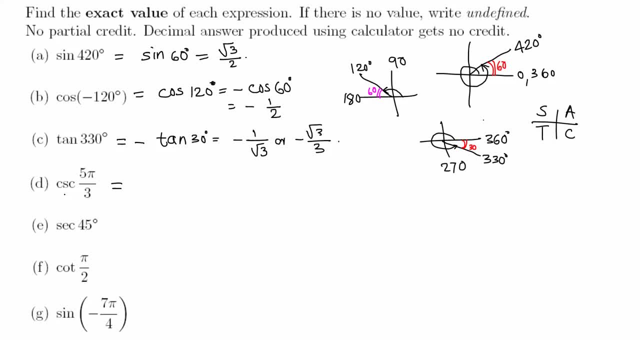 5 pi over 3. okay, cosecant is in fact reciprocal of sine, so 1 over sine. you can go in that way if you are familiar with sine values. so 1 over sine, 5 pi over 3. we can change 5 pi over 3. 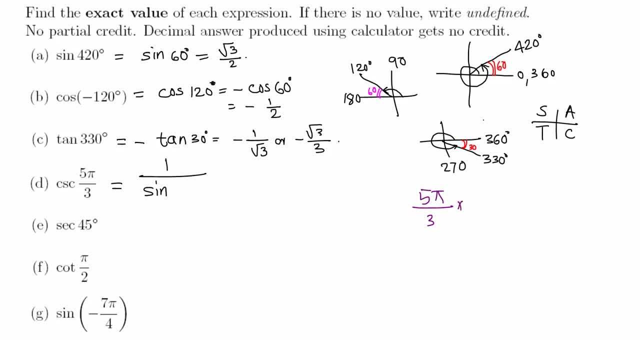 radiance into degree measures. 5 pi over 3, multiplied by 180 degrees over PI, then we get degrees measure. pi pi cancel 3 goes 60 times, and so on 60 times 5, 300. so 5 pi over 3 is 300 degrees. at the same time, cosine is 1. 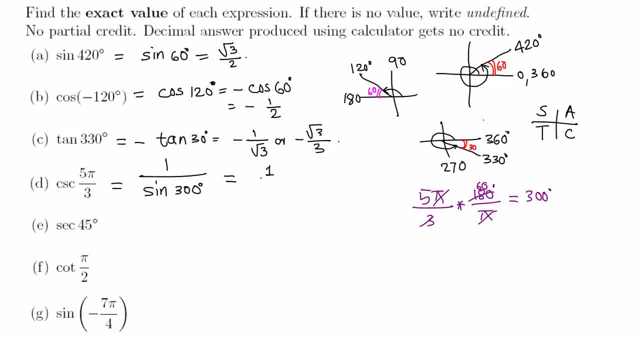 over sine. now that's 1 over. let's find the value of sine: 300. now, 300 degrees is in fourth quadrant. okay, if we try this quadrant, 0, 180, back to 360. this is 270, so 300 is somewhere here, that's 300. so that leaves 300, 360, 60, that's the. 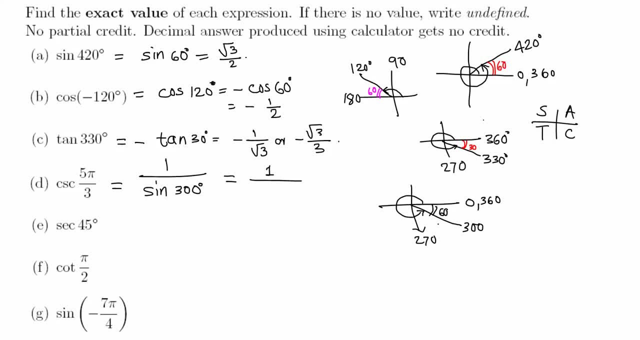 reference angle 300 is in the fourth quadrant. in the fourth quadrant only cosine- and it's reciprocal- have positive values. so sine will have negative value, negative sine of reference angle, that's 60. okay, that is equal to now 1 over negative sine. 60 is a root, 3 over 2. now let's flip this fraction, because 1 divided by this 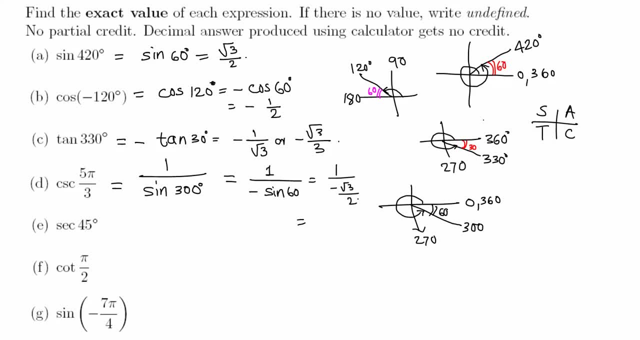 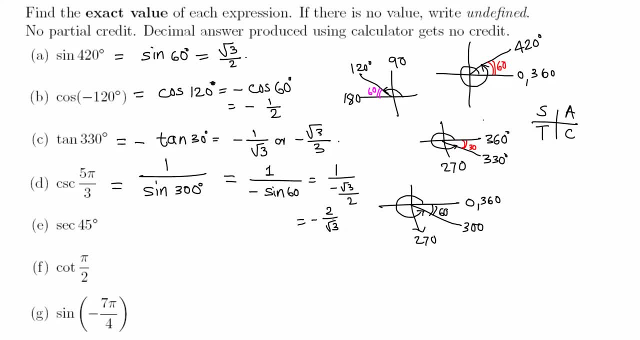 negative in the front: 2 over root 3. this works. if you like to rationalize, you can multiply top and bottom by root 3. okay, next, secant 45. secant is a, the reciprocal of cosine 45 and 1 over. we know cosine 45. cosine 45 is 1 over. 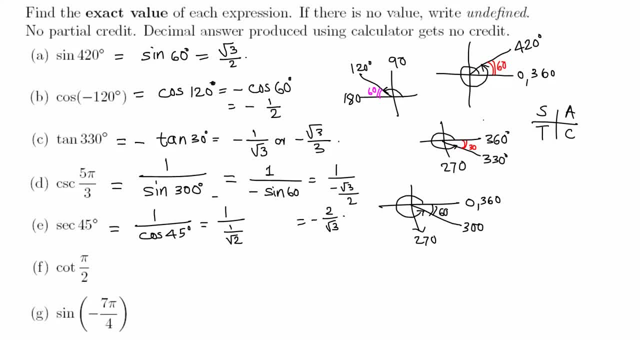 root 2. okay, that is now 1 over 1, over root 2. this division goes into multiplication. this flips becomes root 2, okay, or you just know the value of sine 45, that's the reciprocal of cosine 45 and root 2.. Now next is cotangent pi over 2. 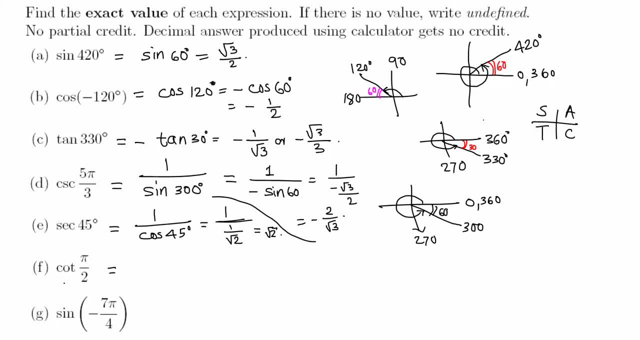 okay. pi over 2. cotangent is the reciprocal of tangent, or cotangent is the ratio of cosine and sine. so cotangent of theta is equal to cosine theta over sine theta. we can go in that way. cotangent pi over 2 is cosine pi over 2 over sine pi over 2 and cosine pi over 2 is 0, sine pi over 2 is 1. 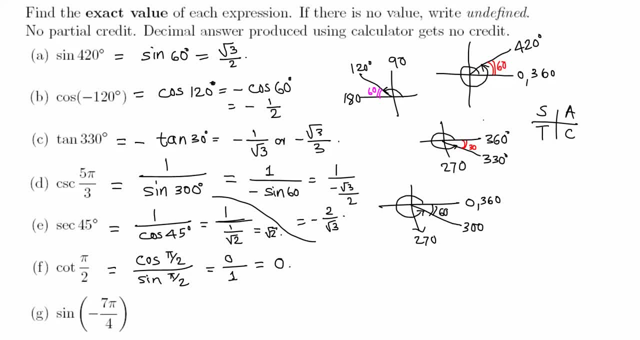 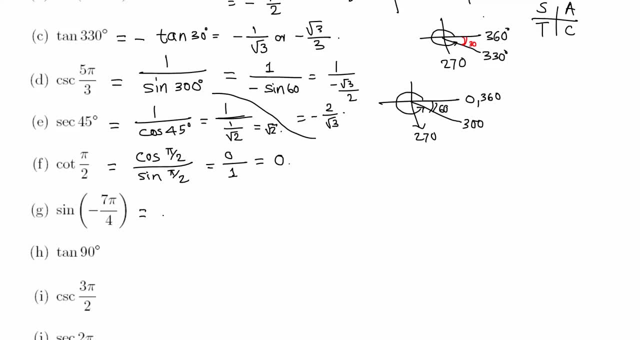 and 0 over 1 is 0, okay. Next. Or tangent pi over 2 is undefined and the reciprocal of undefined is zero, okay. Next. negative 7 pi over 4, sine of negative angle Sine is an odd function, okay. 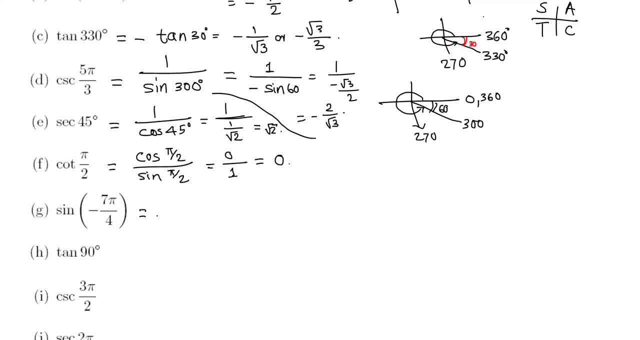 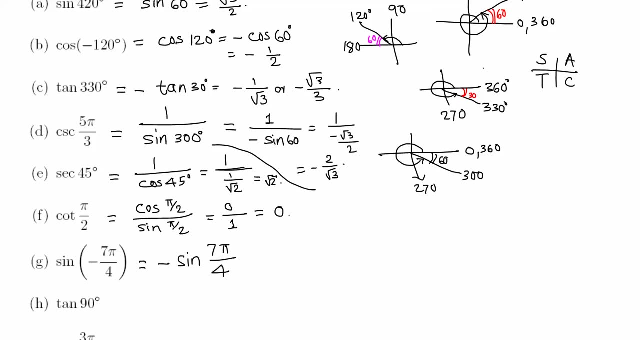 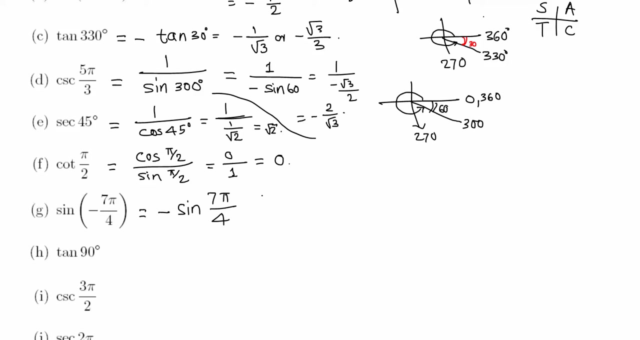 cosine is an even function, but sine is an odd function, so negative of sine. We have seen in part b. cosine is an even function. so cosine of negative angle is positive cosine. But any other sine or tangent sine of negative is negative. sine pi over 4, that's negative sine. If you are not familiar with pi, we can. 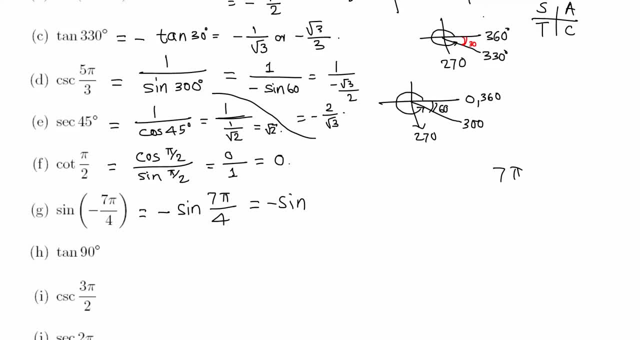 always change this into degrees. So 7 pi over 4. we can multiply by 180 over pi and get the degrees. measure Pi pi cancel 4 goes 45 times. now 45 times seven, 7. use your calculator: multiply 45 times 7, that's 315.. 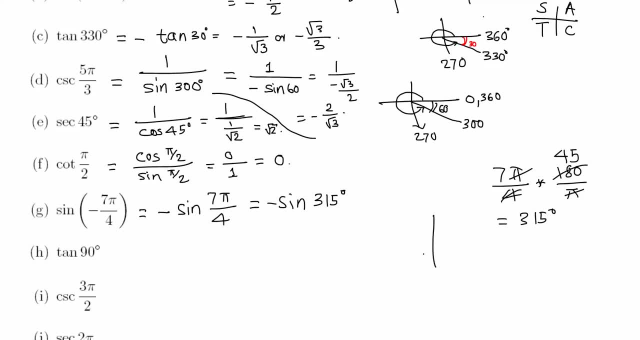 Okay, 315. now let's try to determine where 315 lies. this 360 or 0? this is 270, so somewhere in the fourth quadrant. so 315 is somewhere here, so that we have the reference angle of 360 minus 315, that's 45. 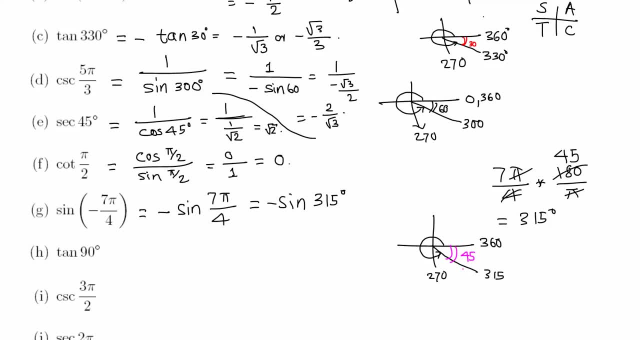 so 45 and fourth quadrant sine will have negative value. sine has negative value and we already have negative and sine will have negative value. negative times, negative will be positive. okay, so this is sine of 45 degrees, because negative again, another negative being in the fourth quadrant. so 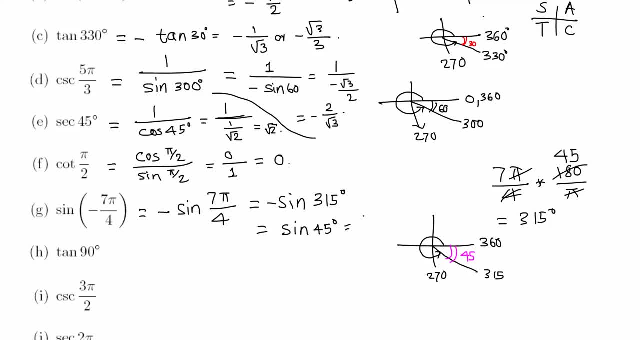 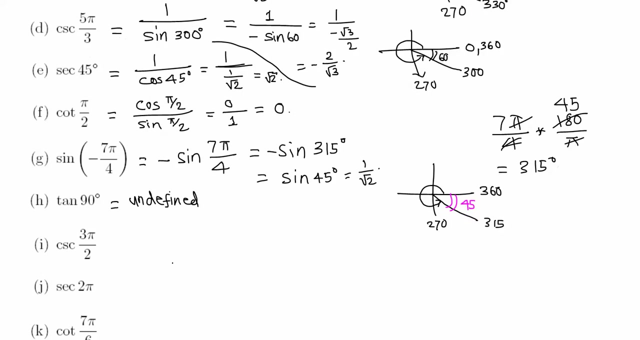 they become positive. sine 45- and we know the value of sine 45, which is same as cosine 45: 1 over root 2.. Okay, tangent 90, that's undefined. you can check in this way: tangent is sine 90 over cosine 90 and 1 over 0. that's undefined. now, cosecant 3: pi over 2, that's same as. 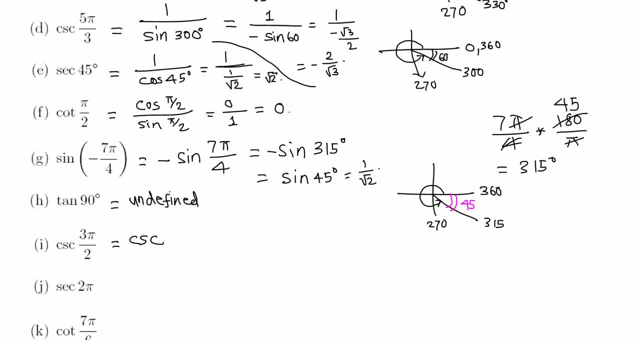 cosecant: 3 pi over 2.. You can change this into degrees. 3 pi is 180 degrees 3 times 180 divided by 2, so that's 270.. And if you are not familiar with cosecant, you can always go for 1 over. 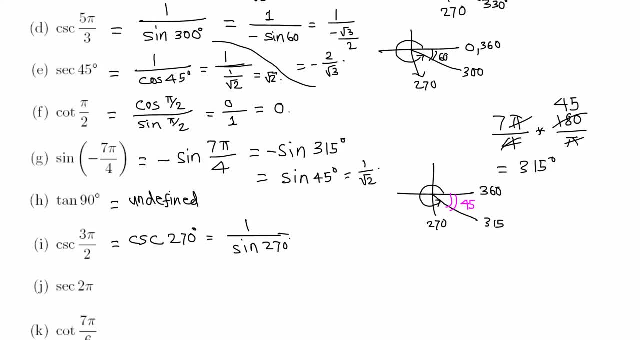 sine reciprocal, half sine 270.. So 270 is in fact the negative y-axis side here. if we take a point, if you are considering unit circle, that will be 0.. negative 1. so cosine 270 is 0, sine 270 is negative 1. 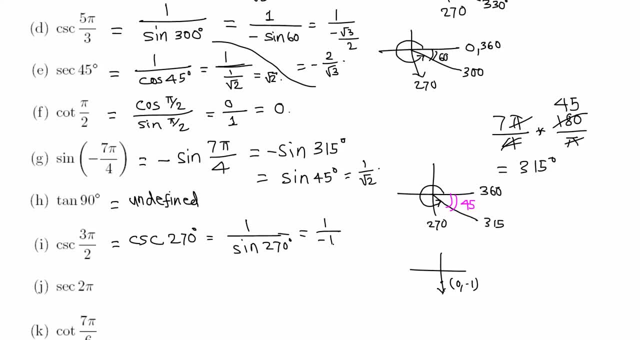 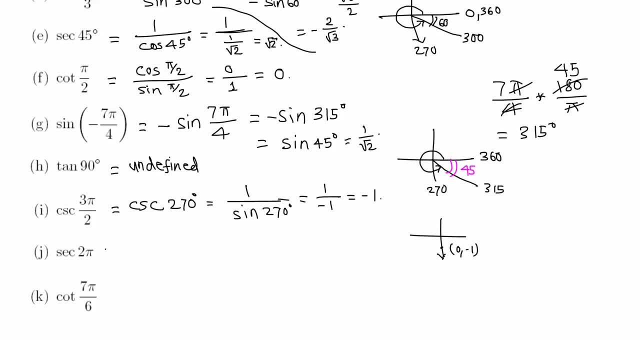 so this is negative 1. so 1 over negative 1 negative in the front, 1 over 1 is just 1.. Okay, next, secant 2 pi. the secant 2 pi is 360 degrees, if you want to change into degrees, and 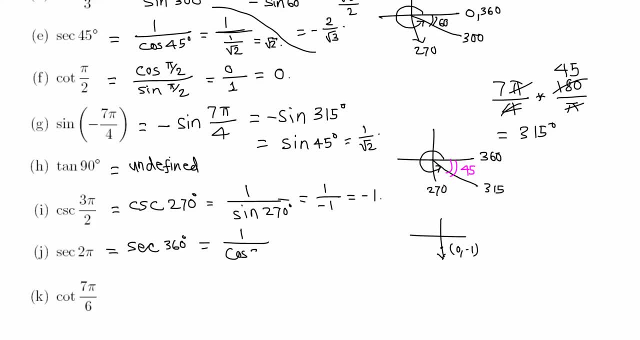 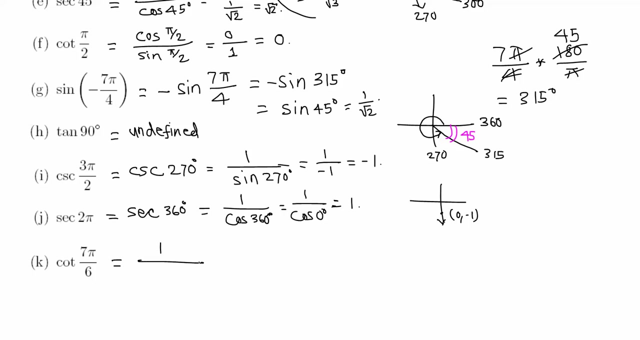 secant is reciprocal of cosine cosine 360. Okay, and, by the way, 360 is same as 0 degrees cosine 0 and cosine 0 is 1. 1 over 1 is just 1.. Cotangent: 7, pi over 6. cotangent is 1 over tangent, or you can go for cosine over. 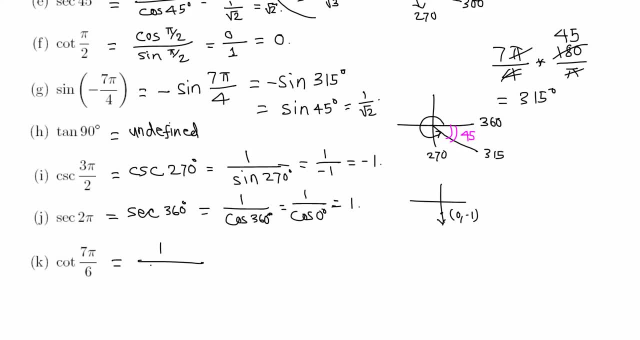 sine, your choice, or you can just find the value of cotangent directly. so I'm going to go for tangent. 7 pi over 6. I want to change that into degrees: 7 pi over 6. multiply or replace pi by 180. same thing, 180 over pi, pi cancel. 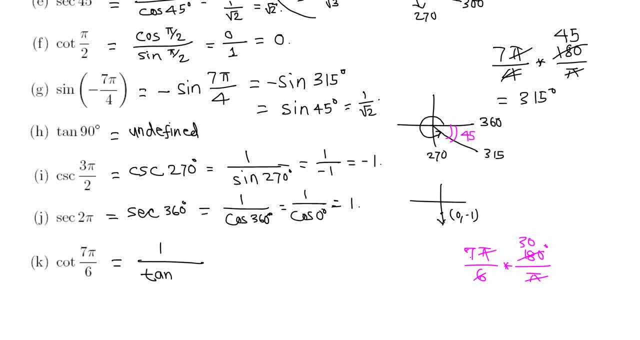 6 goes 30 times 30 times 7, 210, so that's 210 degrees. so that is 1 over tangent 210. 210 that's 180, 90, so 270. so 210 is in the third quadrant. start from this positive x side, that's 270.. 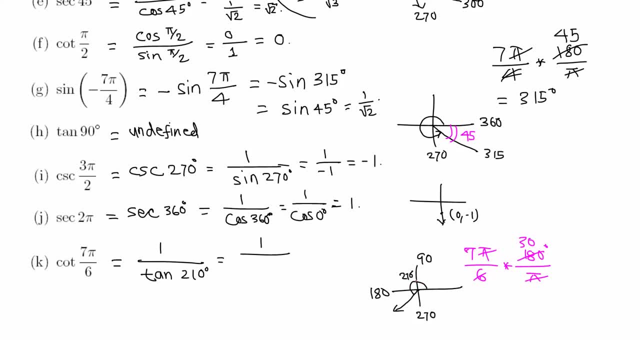 So the reference angle will be then: uh, that's 210, right, 210. 210 minus 30, 210 minus 180, that's 30.. 30 is the reference angle. so, tangent 210 is 10, plus or minus tangent the reference angle, that's 30, and we are in third quadrant. 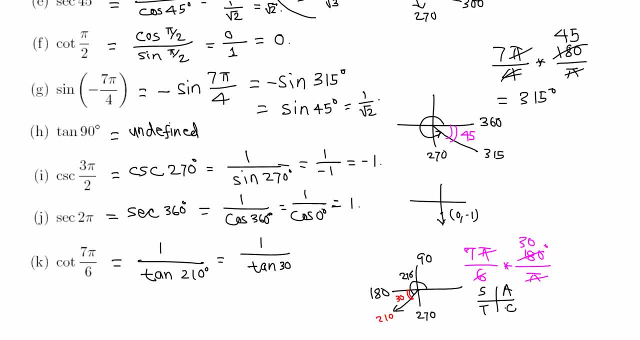 if you want to go with this rule. all students take calculus in the third quadrant. tangent has positive value, so plus and 1 over. we know the value of tangent 30. tangent 30 is 1 over root 3.. So 1 over 1 over root 3. change this division into multiplication. 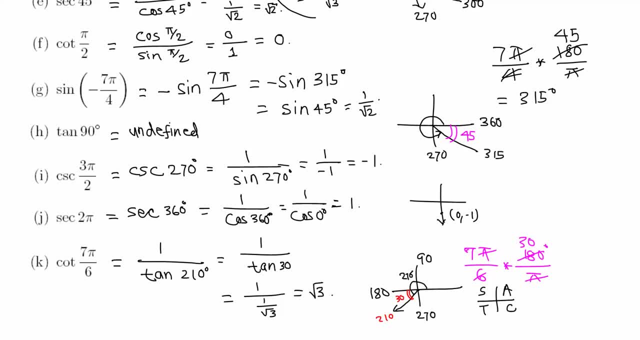 1 over root 3. this flips. this becomes root 3 final.